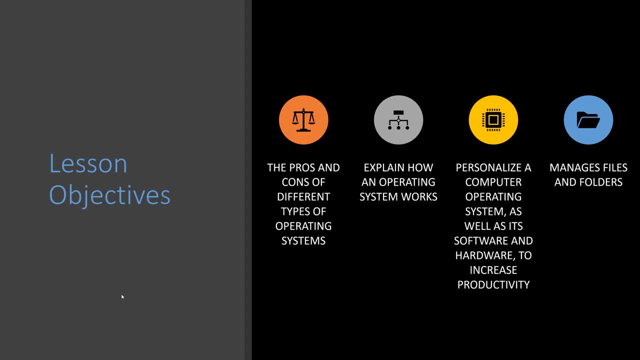 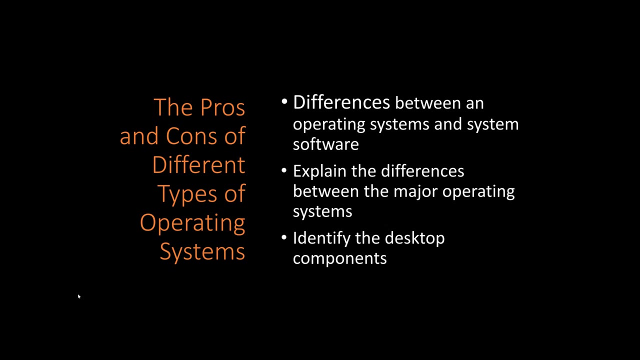 how an operating system works, how we personalize the operating system to better meet our productivity needs and then, finally, how we manage files and folders. For this section, the outcomes are. I'll demonstrate the differences between operating systems and system software. explain the differences between the major operating systems. 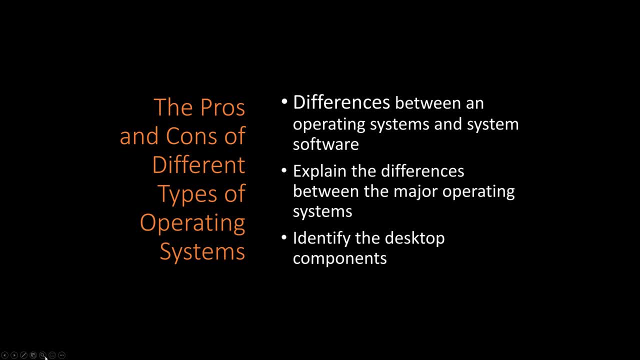 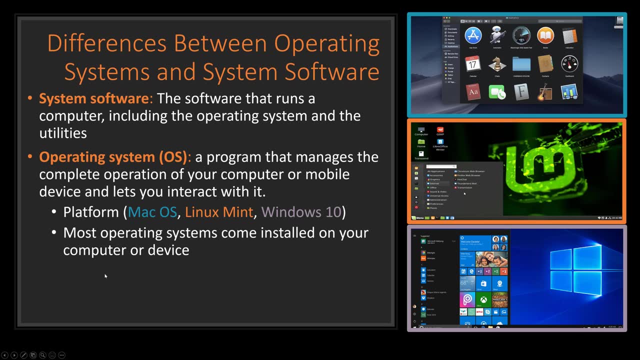 identify specific desktop components that are unique to primarily client operating systems. So, as we look at this, the differences, first of all, are what computer it runs on, what hardware. We've talked in previous episodes. We've talked in previous videos in regards to processors, memory, etc. 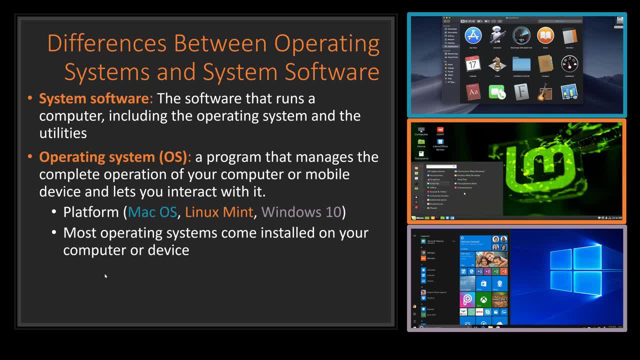 And different operating systems are going to use different resources, meaning the old Apple Mac operating system required a proprietary CPU in order to run. Now they've since switched to a standardized Intel CPU Intel chip format, which means it will run on Intel chips. 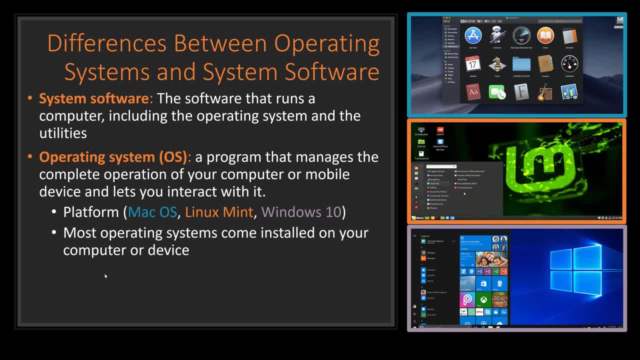 However. However, now they're going back to manufacturing their own proprietary CPU. So you want to make sure you know that you're meeting the hardware needs of the operating system you choose. Now, here on the right, I've given you three of the primary operating systems for client, which means desktop, laptop. 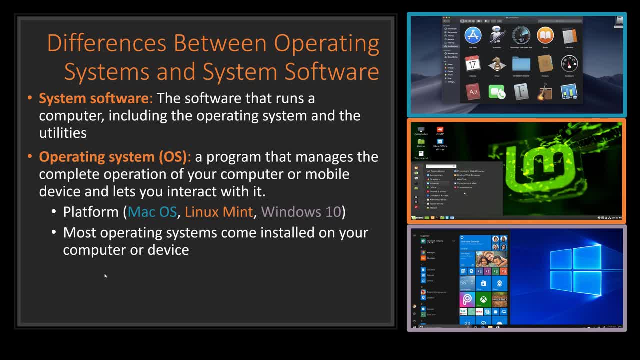 what you're used to using as an end user system At the top right in blue is going to be the Mac operating system. Of course, this is Windows based. It is proprietary, meaning that you know they have license over it. 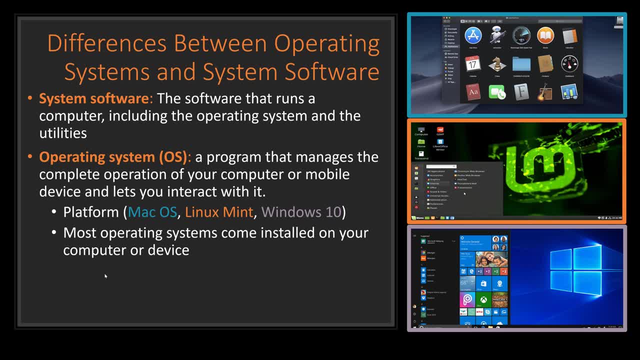 You must buy a license to use it. Then there's Linux Mint. Linux is an open source. Unix, Linux- you've probably heard those terms. Those are open source. That means there's an entire community that programs the operating system. Now what happens is communities will get formed, like you know, the community that runs Linux Mint- and they'll specialize in creating an operating system. 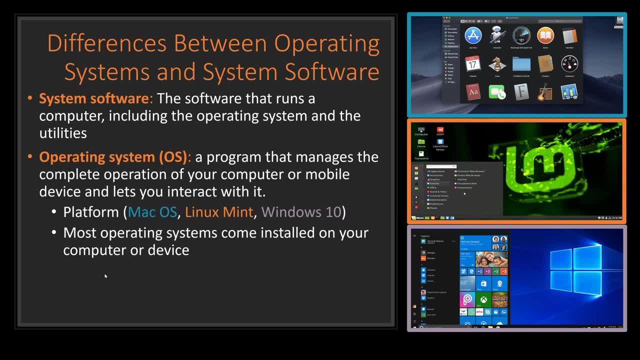 And they'll specialize in creating an operating system, And they'll specialize in creating an operating system from the Linux kernel that you can run. So an example here is Linux Mint, Another might be Ubuntu- or Ubuntu, depending on how you say it- et cetera. 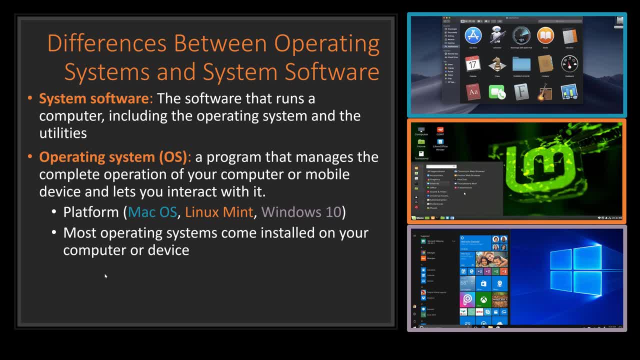 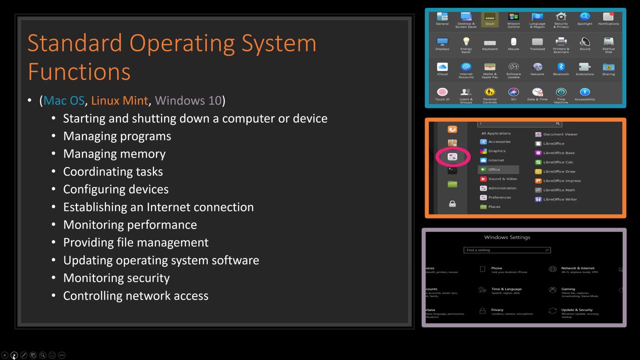 And then, of course, you're probably familiar with Windows 10, which is manufactured by our program, by Microsoft Corporation, And that's down here at the bottom. I'm giving you an example of a Windows 10 operating system. We're looking at the desktops of these different operating systems. 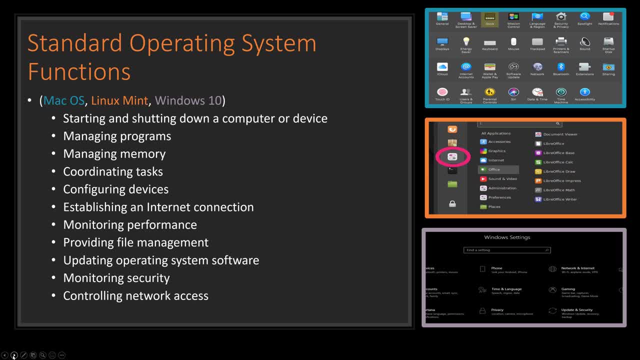 Now, what do we do with an operating system? Well, as mentioned in a previous video, this is the first piece of software. Well, let me be careful here. This is the first piece of software that we're installing, But realize that in our system is a ROM chip that holds the BIOS, the basic input operating system. 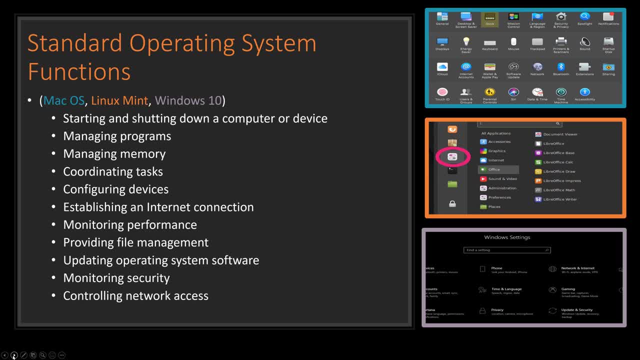 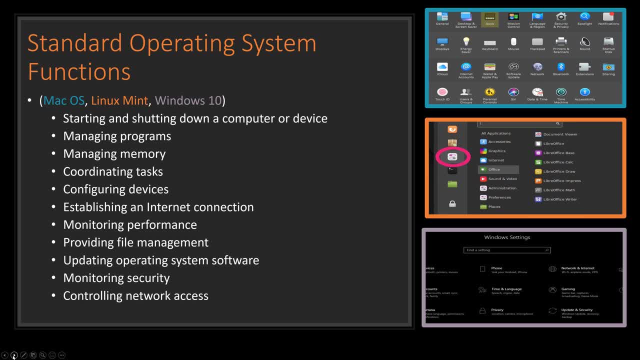 It is the, it is what runs to allow us to load the operating system software that we want to use from our computer Through the processor into the memory so that we can use it. Okay, so what we can do with these, you know. start, shut down a computer device. you know, with the operating system we can manage programs: who can use what program, how that program is run. 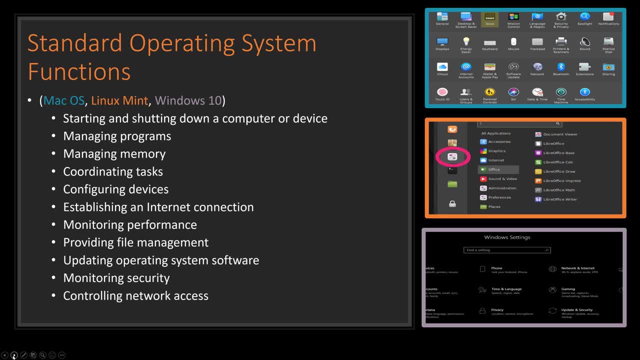 So maybe there are certain programs that need to be run with administrative levels. Okay, that can be risky from a security standpoint, but we can right click and say run as administrator or configure it To always run with higher level privileges. Okay, we can manage memory, we can coordinate tasks. 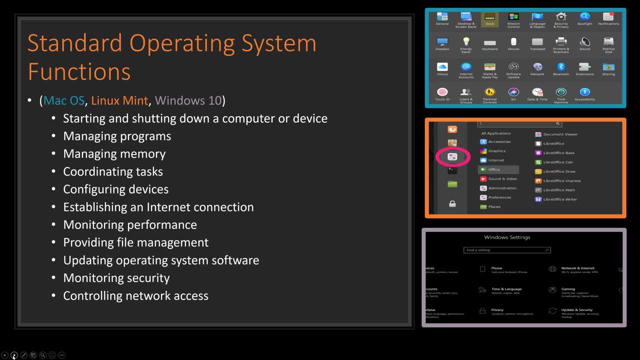 By coordinating tasks, realize we can also remove software we are not using. We can remove services that we are not using or close services so that the limited resources we have on our computer can be utilized to maximize performance as we use it. So, for example, as I am recording this video, 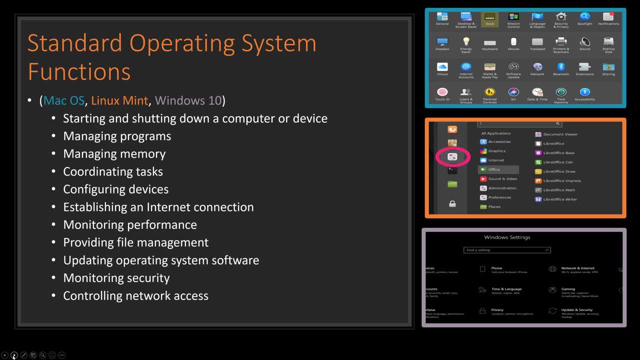 So, for example, as I am recording this video, I go ahead and shut off things that I don't need right now. I go ahead and shut off things that I don't need right now So that all the system resources can go to that. 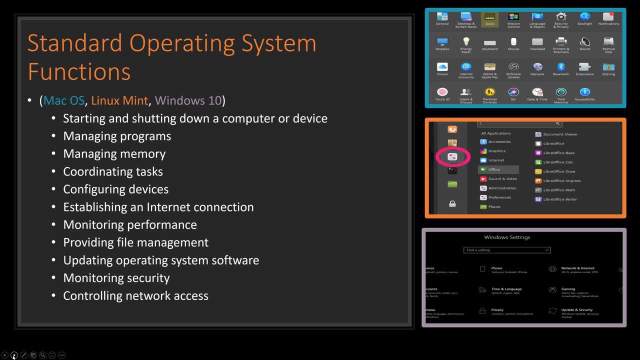 Once I am done recording, I then go in and do post production, Where, if I make a mistake that I want to get rid of, I will remove the audio, remove that portion of the video, shrink it together And then, finally, I will produce it and stick it up to YouTube, for example. 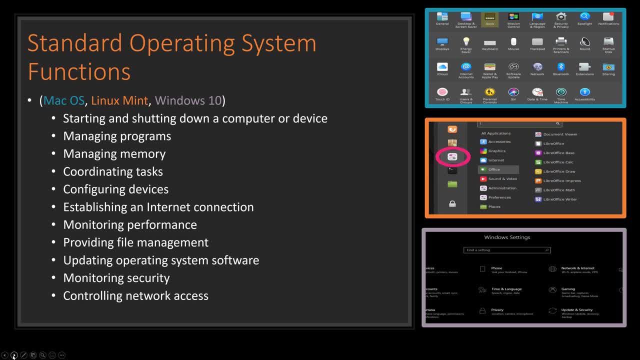 Or it might just be a video for my class specifically, So I can do those kind of things as well. I can monitor performance so I can see what is going on. So if my computer seems to be running really bad, So I can monitor performance, so I can see what is going on. 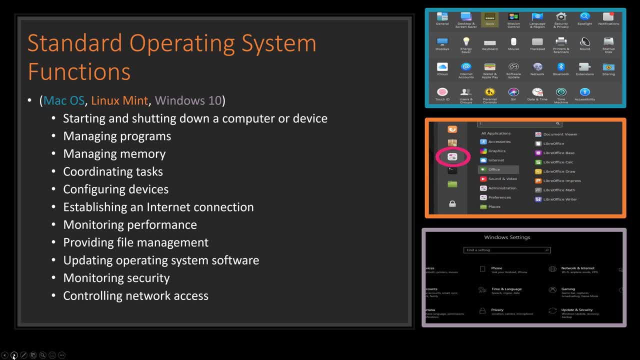 So if my computer seems to be running really bad, So I can monitor performance, so I can see what is going on. So if my computer seems to be running really bad, So if my computer seems to be running really slow, what I might do is go out and look at the network performance. 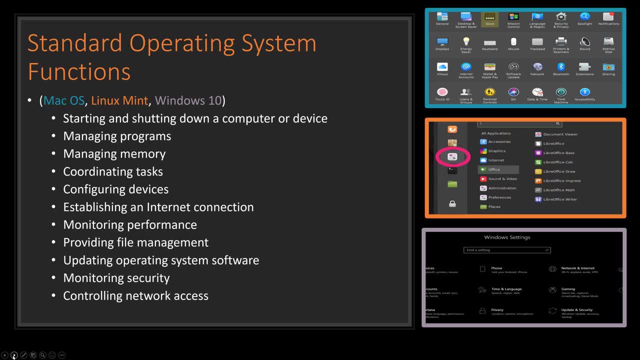 And see how much data is transferring from my computer maybe out to the network or out to the internet, And see how much data is transferring from my computer maybe out to the network or out to the internet. So by doing that I could see if maybe there is a virus or something that is, or spyware, that is using my system resources. 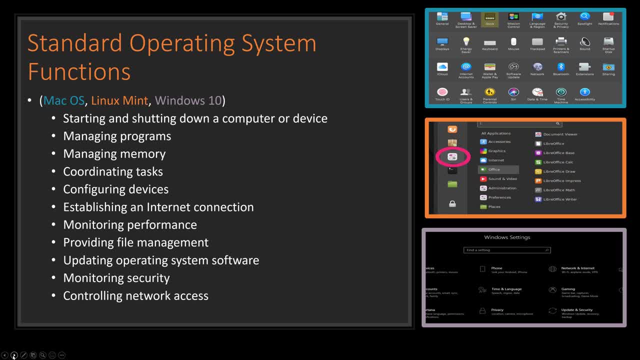 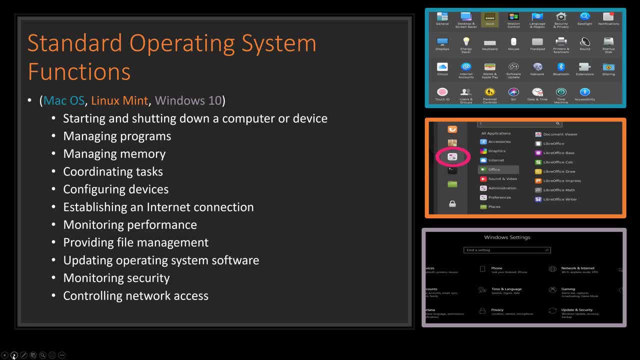 And it is constantly sending information out or using my computer to process things that I am unaware of. Provide file management, of course, as we start putting everything onto the computer. Provide file management, of course, as we start putting everything onto the computer. Provide file management, of course, as we start putting everything onto the computer. 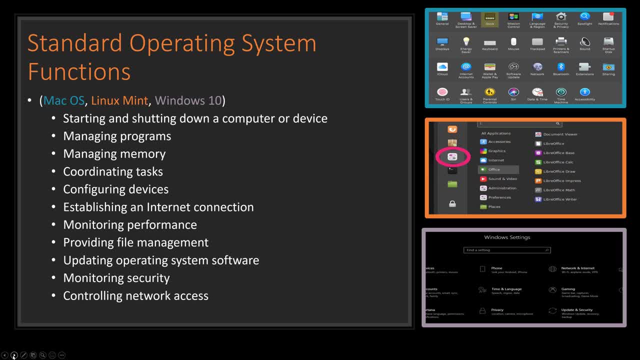 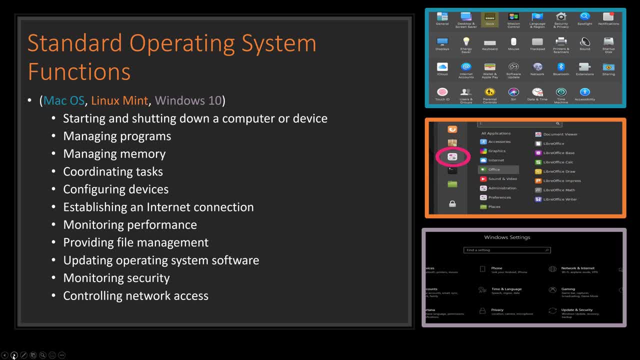 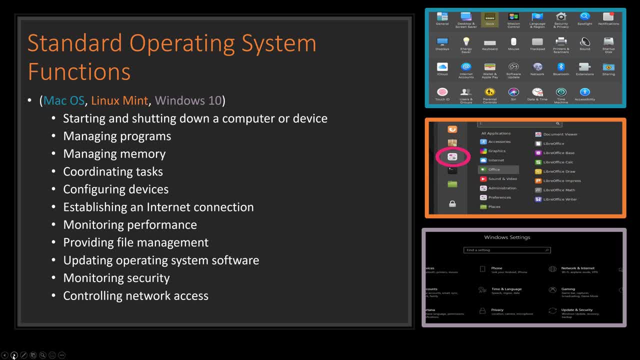 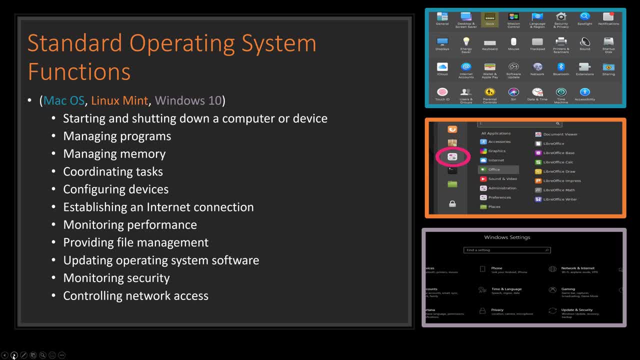 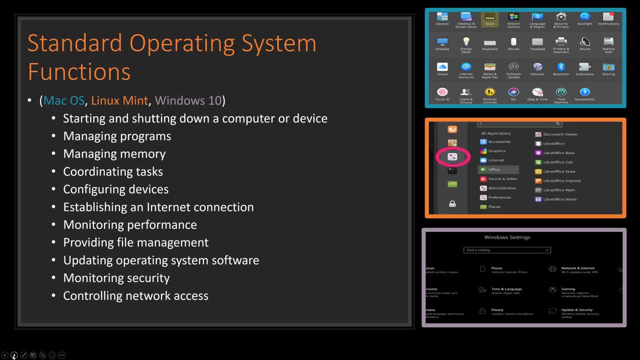 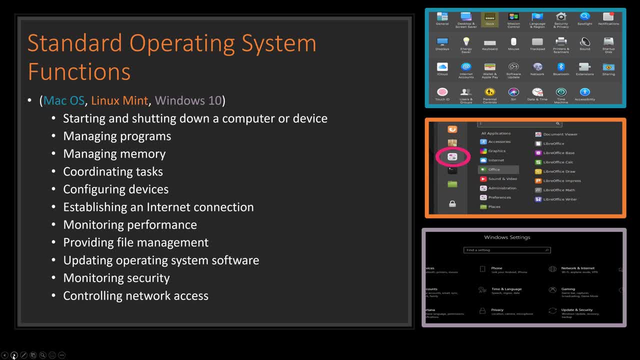 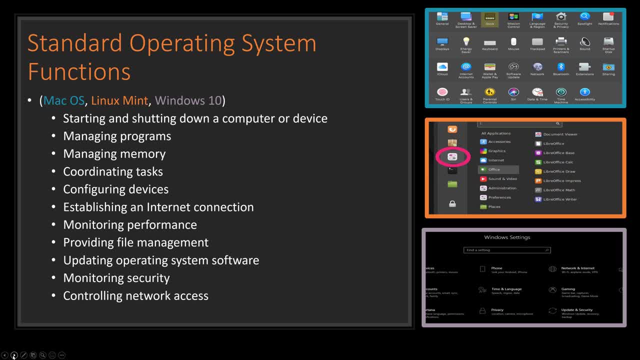 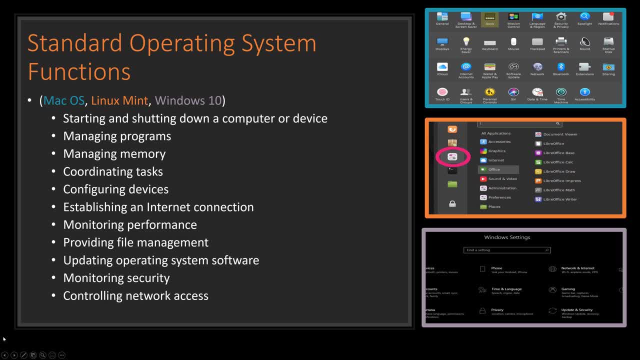 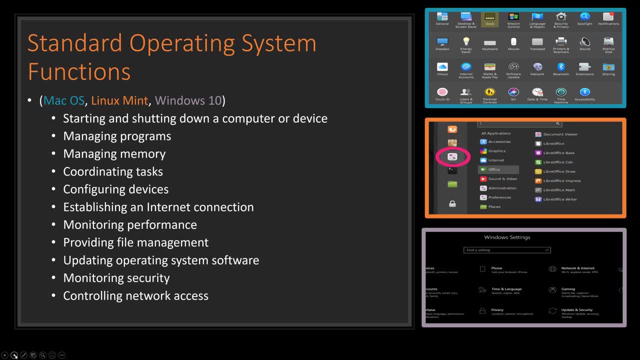 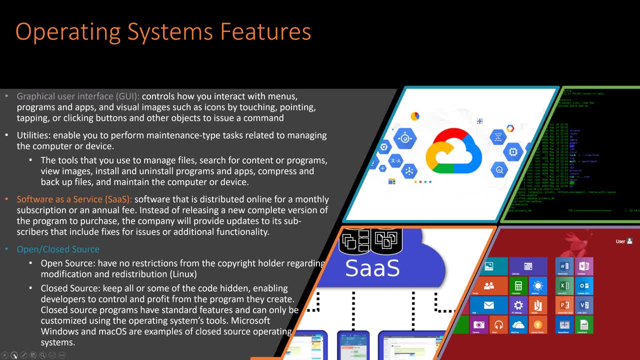 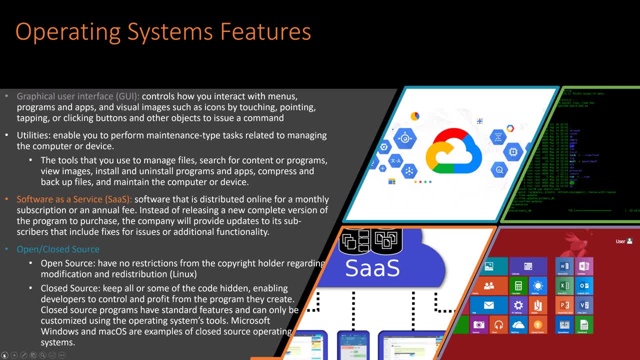 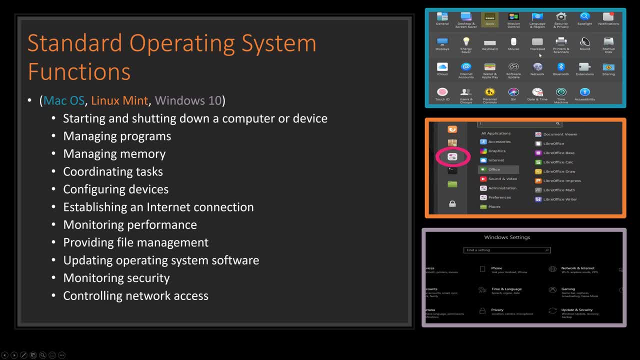 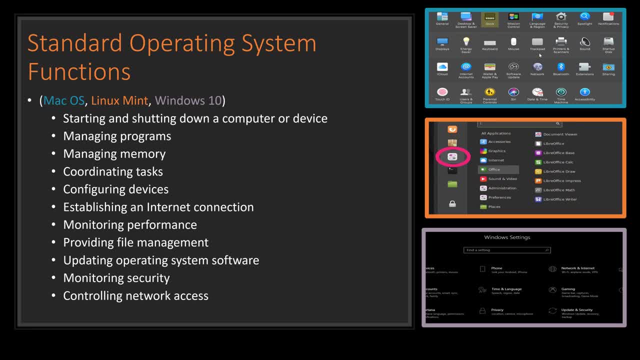 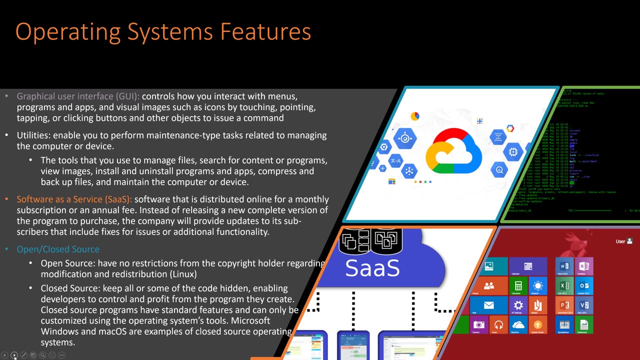 operating system or the system functionalities are for Mac, system functionalities for Linux, Mint and system functionalities for Windows, Moving on. so operating system features. Normally today there's two types of operating system controls, Now what we're used to back. when computers first came out, all of their operating systems were what was called command. 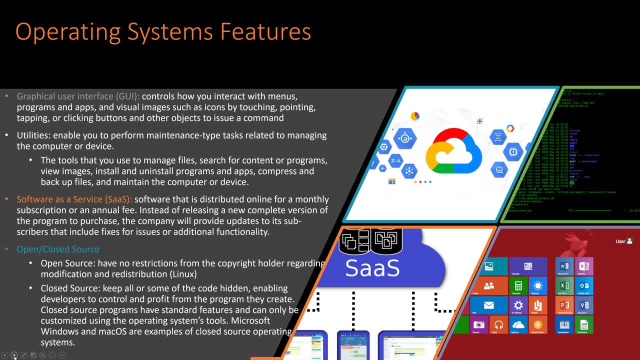 line interface. And the cool thing about command line interface was that we didn't have the extensive processing power in order to manage a graphical user interface. So I've read that upwards of 60 to 70% of the resources of a computer go to producing the graphical user. 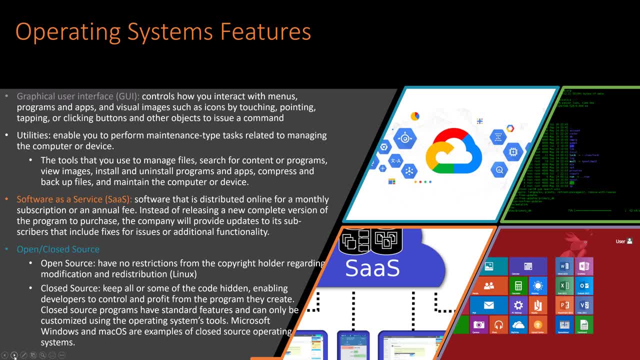 interface. Now, of course, that makes it easier for end users because they can just click and go versus having to go in and type a command. Okay, So examples of this real quick. So here down here in the right, this is a graphical user. 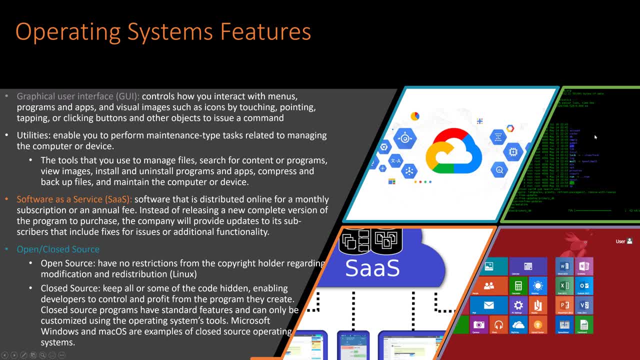 interface for Windows 10.. And up here is a command line interface: okay for a Linux operating system. So although- and we'll talk about this- Linux does come with graphical user interfaces on the client side, a lot of times it's much more efficient to get rid of the 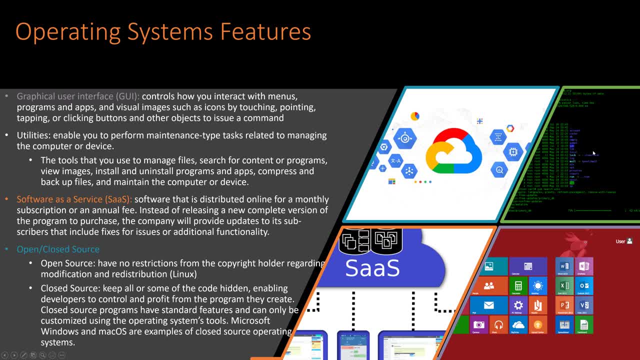 this processing power and use it for whatever task the computer's going to run, instead of a graphical user interface. Now, what that means is we have to learn commands on how to do things, including how to connect it to the internet via a command line interface. Also today, there's the 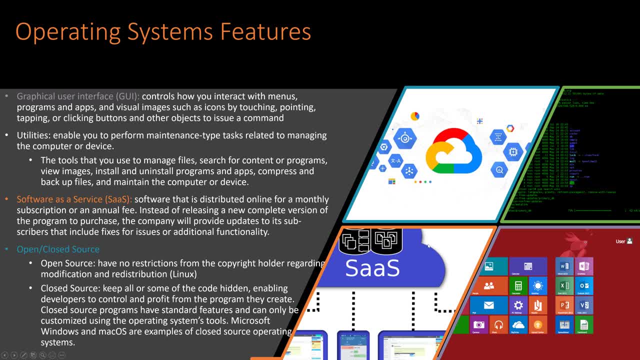 opportunity for software as a service. Now I'll give you an example down here. If you notice, this is representing the cloud and these are different devices. Now the cool thing with software as a service is, if it's programmed correctly, it's going to use an internet browser that you're going to interact. 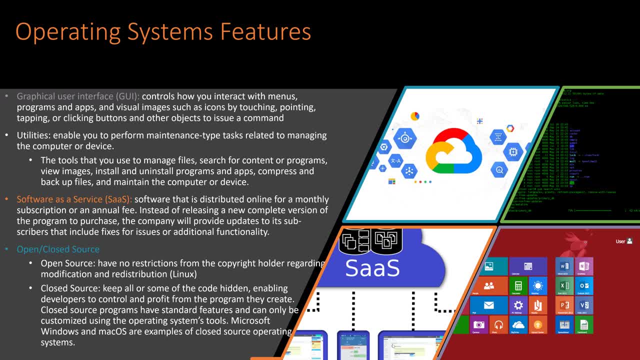 with the browser in order to manage the software. Let me give you an example of this. Some of you may be familiar with QuickBooks. Well, QuickBooks is actually an accounting software that started out with. you bought it, you installed it on your computer. Now you can get QuickBooks where your 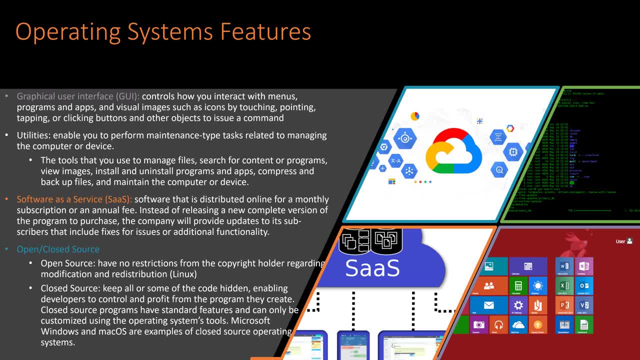 files, your data, is stored in the cloud and QuickBooks becomes responsible for it. Now you can get QuickBooks where your files, your data, is stored in the cloud and QuickBooks becomes responsible for it. Now you can get QuickBooks where your files, your data, is stored in the cloud and QuickBooks becomes responsible for it. 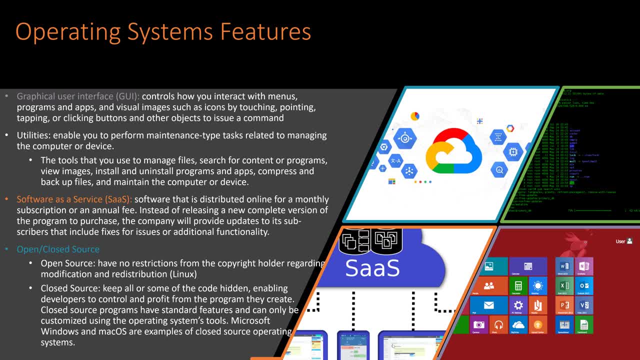 Now you can get QuickBooks, where your files, your data, is stored in the cloud and QuickBooks becomes responsible for it. But the cool thing is now, if I'm on my smartphone, I need to enter something in my QuickBooks and I'm connected to the internet. I can do it. 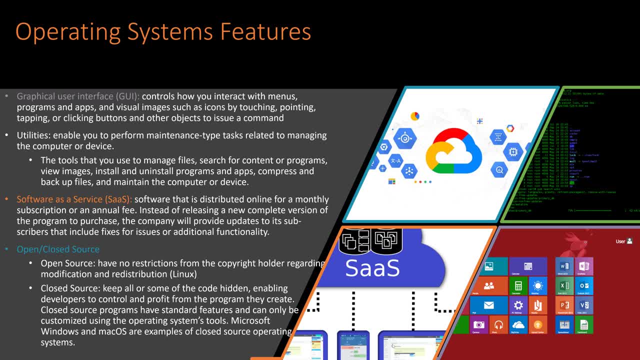 I don't have to be on the computer that's hosting that particular version of QuickBooks. I don't have to be on the computer that's hosting that particular version of QuickBooks. We've got a ton of software as a service now. We've talked about storage as a service, email as a service. 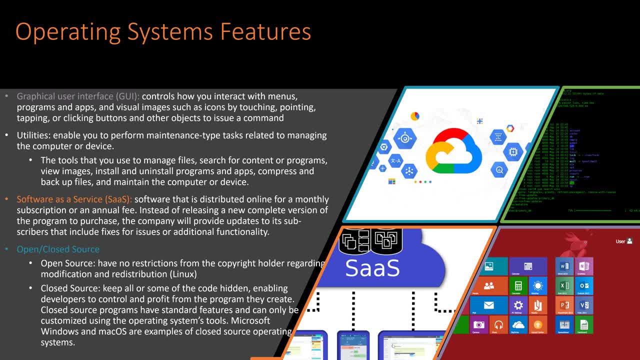 Some of you are probably familiar with Outlook Web Access. That means your employer or your college is no longer running an email server locally. Some of you are probably familiar with Outlook Web Access. That means your employer or your college is no longer running an email server locally. 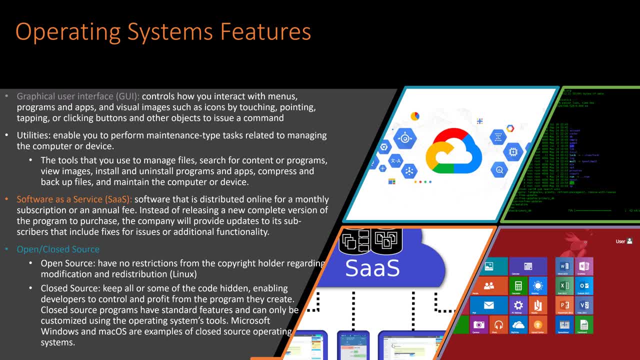 They're using Microsoft's Office 365 as a service. Now, finally, there's open and cloud source. The idea behind this is that we can put up our own servers to do things meaning in Microsoft Azure, which is their cloud environment. 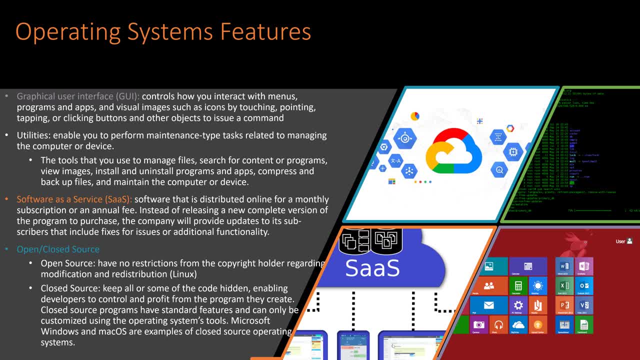 I can put up a server to do something in the cloud that anyone can access or that limited people can access, Even though it's in the cloud. realize I can configure it to where only people in Microsoft, My network, are able to get out to that cloud resource and use it. 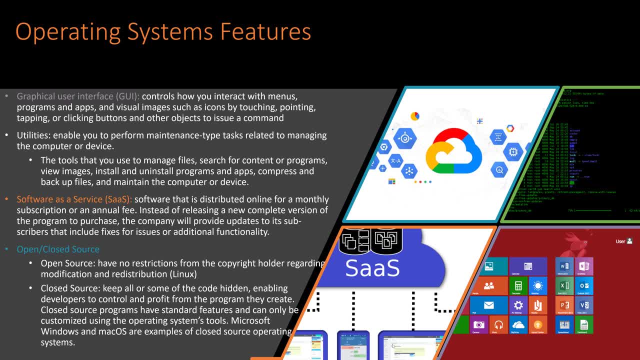 So we see a lot of this with email. We definitely. you know it's been the standard for web pages for decades now. where a web server- usually Unix- is programmed, The Unix operating system is installed on the server, The developer develops the website and everybody is able to access it. 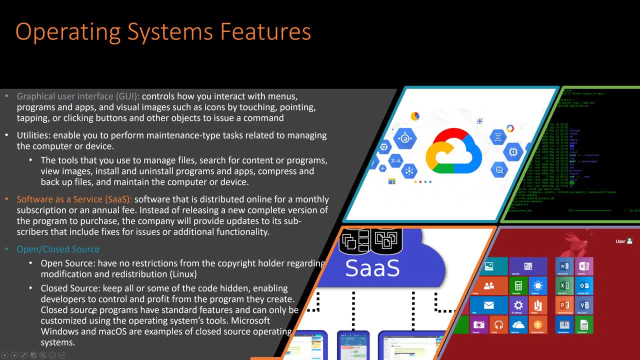 And the cool thing is there tends not to be a great cost with that, versus when you're doing Azure, When you're using Microsoft Azure, When you're doing Amazon, you're paying for the licensing of the operating systems. if you're installing operating systems that indeed need to be licensed. 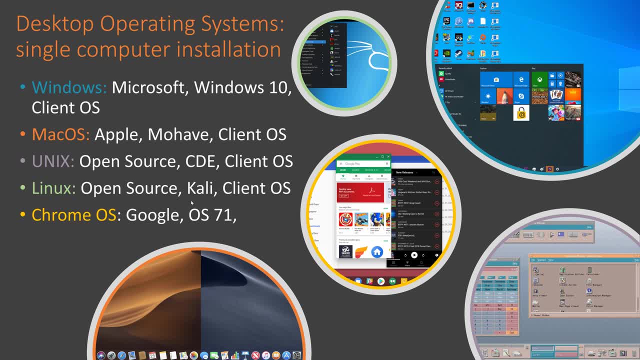 Now some quick examples of some client operating systems. These are the standard ones that we see today, including I threw in a Linux that you may not be familiar with. So Windows- I've already said it's Microsoft product. Windows 10 is a current OS and it is a client OS. 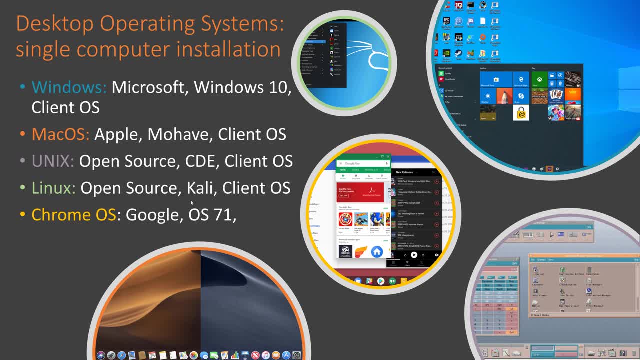 OS means operating, So it is the operating system we would find on our desktops or our all-in-ones or whatever Mac OS. you're probably familiar with it. So on, you know, MacBooks and et cetera, it's the OS. 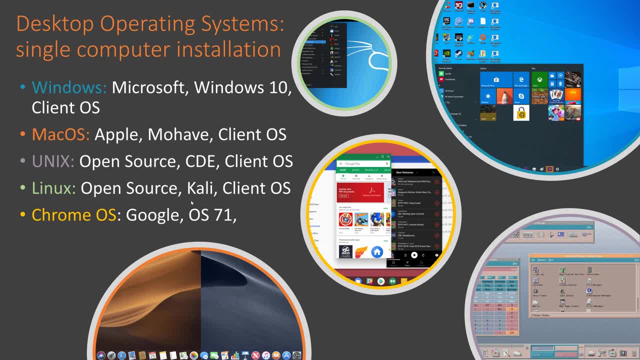 It's Apple. Oh, by the way, Windows proprietary: Okay, I can't run it for free. Windows programs it, I got to pay for it. Mac proprietary by Apple: Okay, Even more proprietary, because I can actually buy Windows operating system and put it on an independent computer. 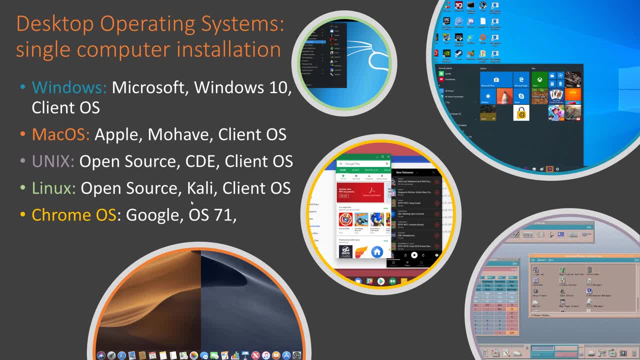